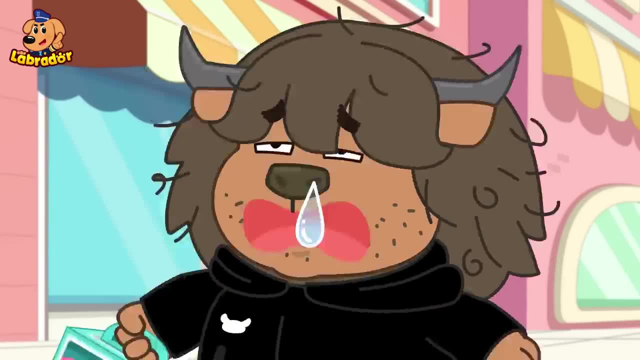 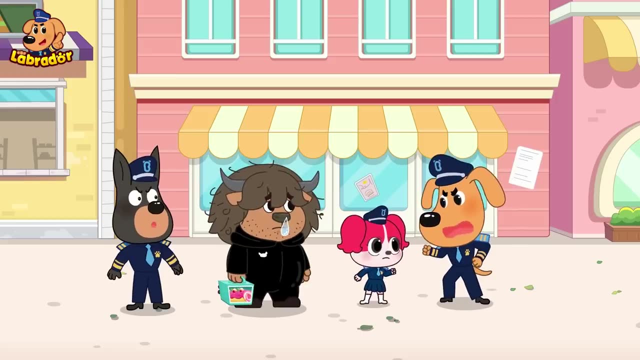 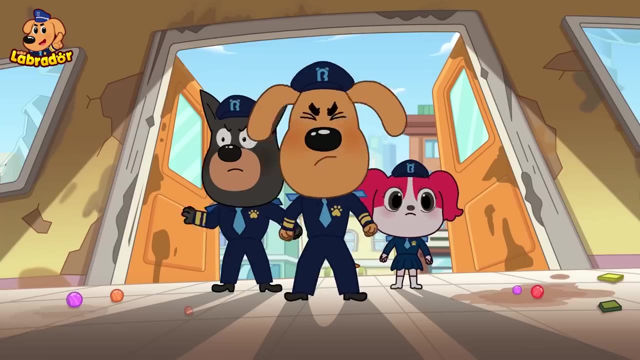 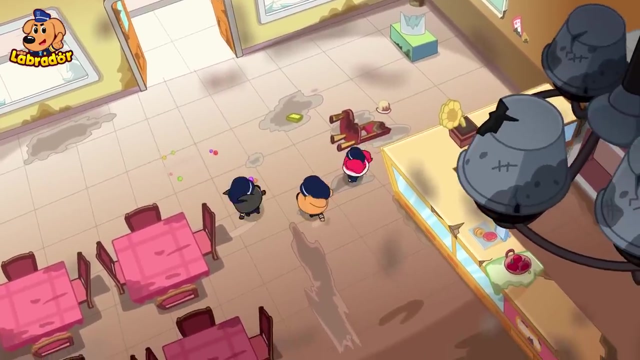 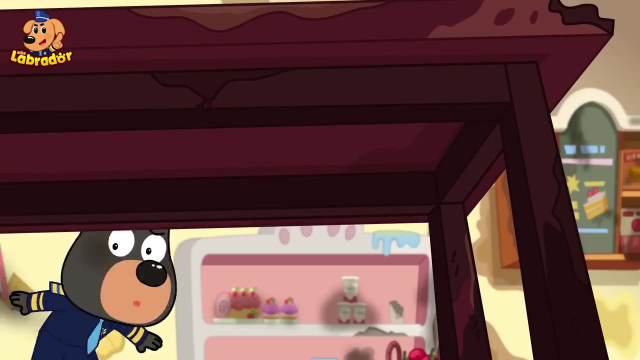 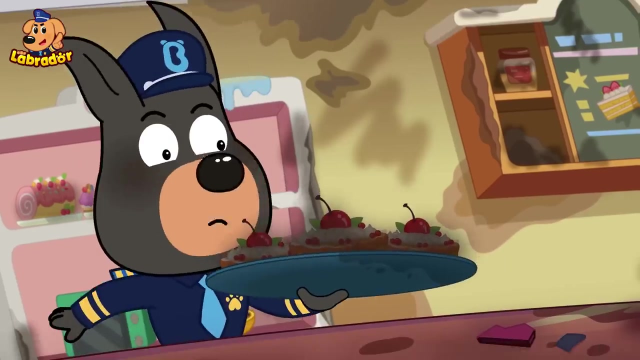 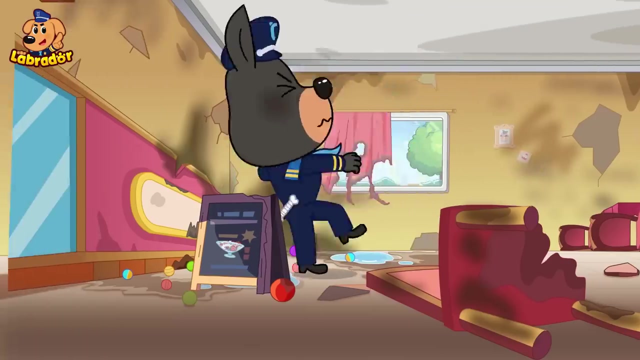 Because I have a cold. Sorry, my mistake. I think we need to investigate the scene. Let's go. The shop is severely damaged. We need to be careful. Okay, Watch out. This is the cake. I couldn't finish. Watch out. 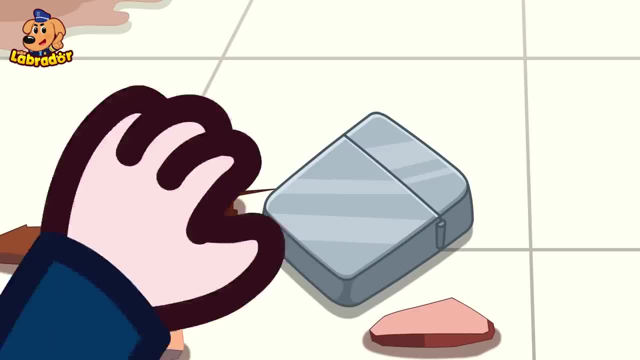 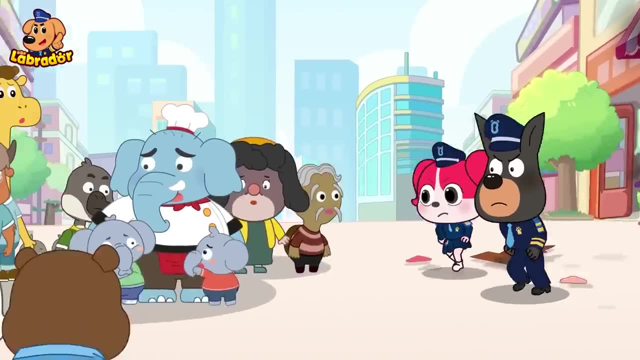 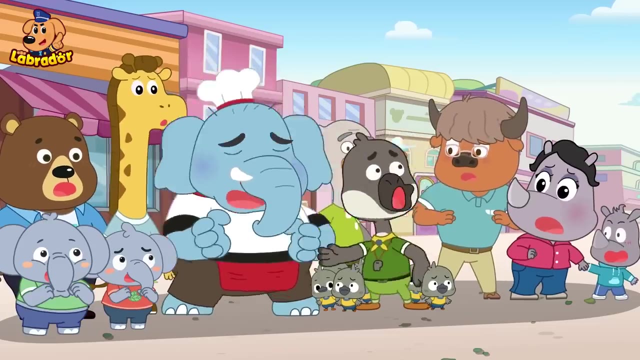 Dobby, are you okay? I'm fine. A lighter, It's Mr Wild Goose's. We need to find him right now. Mr Wild Goose, is this your lighter? A lighter, Hey, did you start the fire? 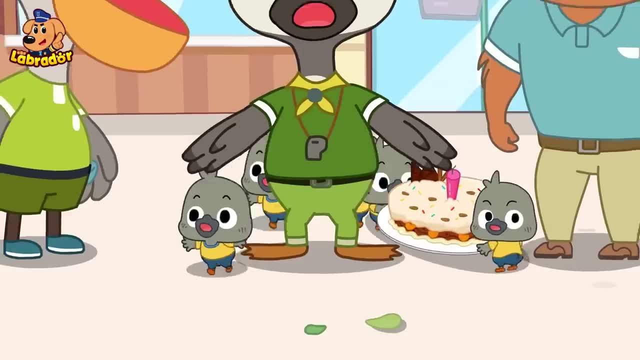 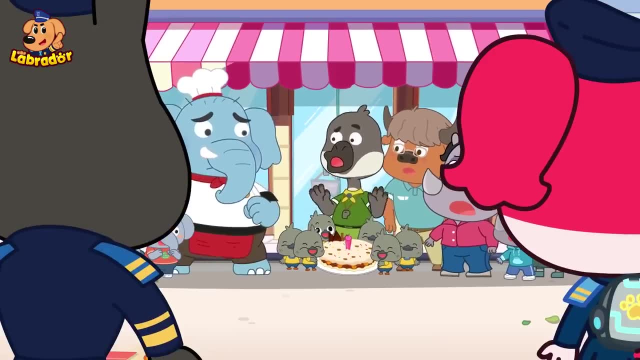 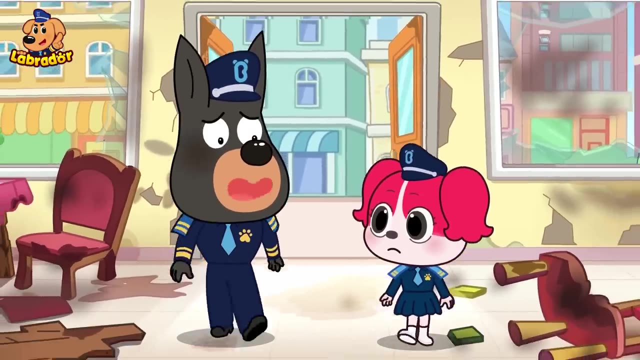 What? No, I didn't. Daddy was going to light the candle on our birthday cake, But we haven't lit it yet. Oh, I'm sorry, I misunderstood you. Another dead end. Phew, We haven't even found out who started the fire. 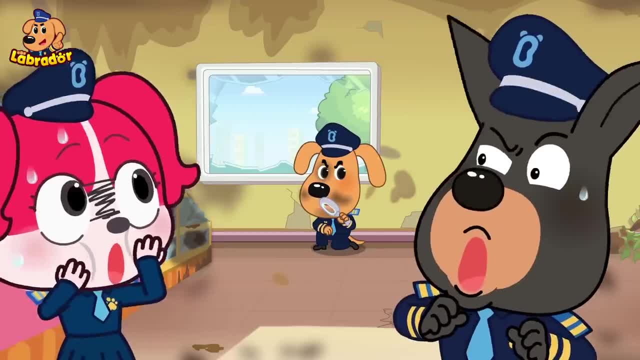 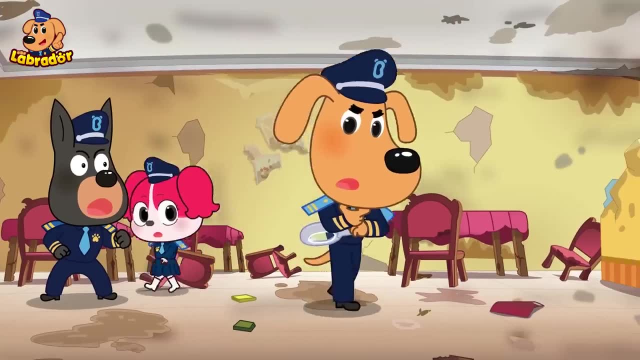 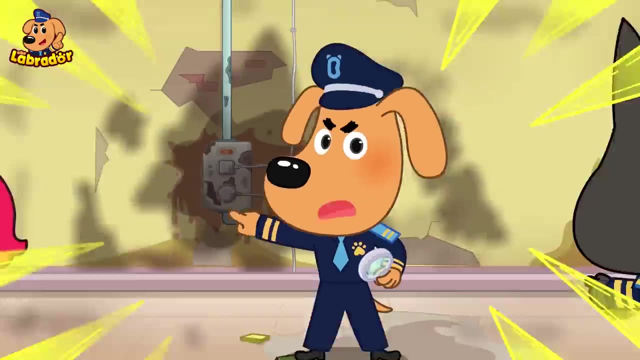 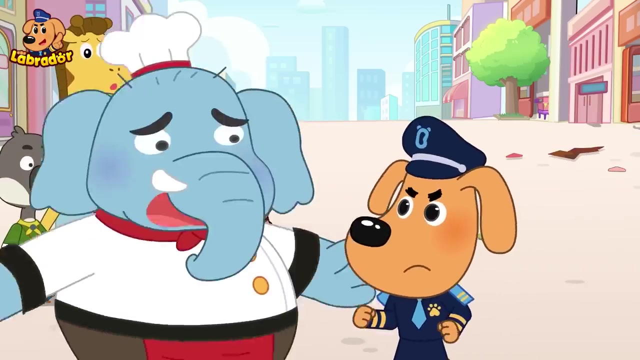 Phew, I found something. Huh, Sir, your face. Huh, Based on evidence, this is where the fire started. Huh, I found the cause of the fire. Sheriff Labrador, did you find out anything? Yes, The Elephant Brothers over there started the fire. 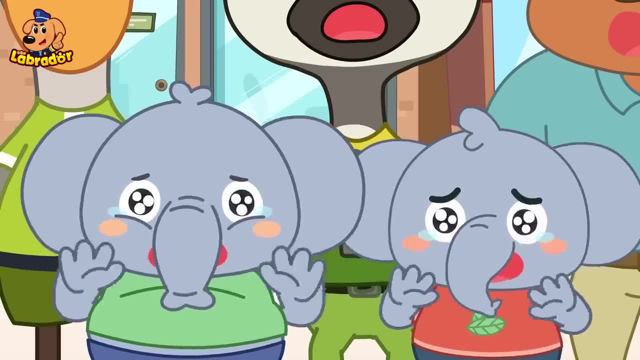 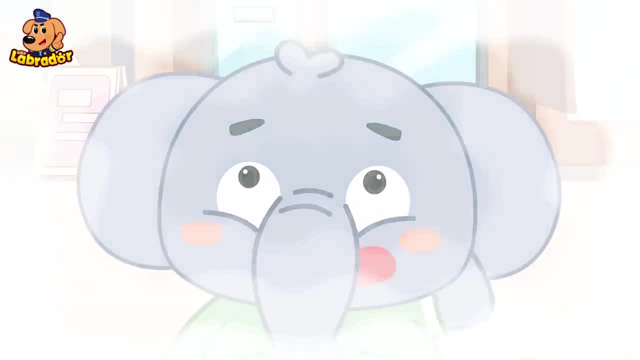 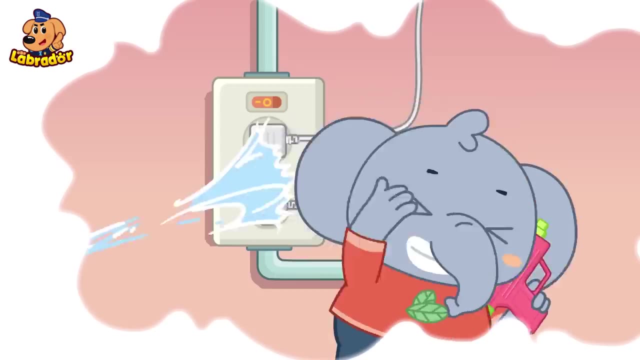 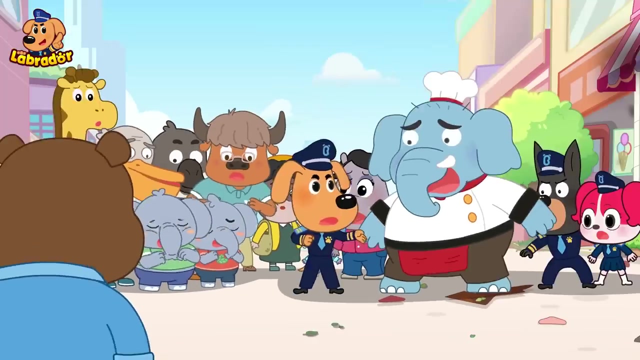 What My children, Not us, We didn't do it. Kids, you were playing with water guns, right? Yes, We were playing cops and robbers. Hey, stop running. They sprayed water onto the electrical outlet, which caused it to short-circuit, and then the fire.